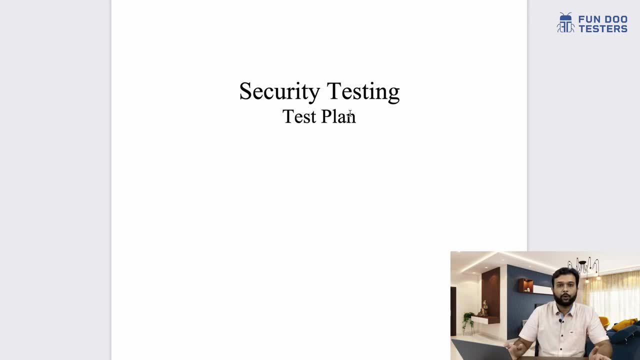 similar document for the functional testing or automation testing or api testing. so first thing is we are going to mention title: what is a test plan and here we can place a company logo and who are going to create, like that we can do. and first second part is index. so index what are the points or what are the things we have covered. 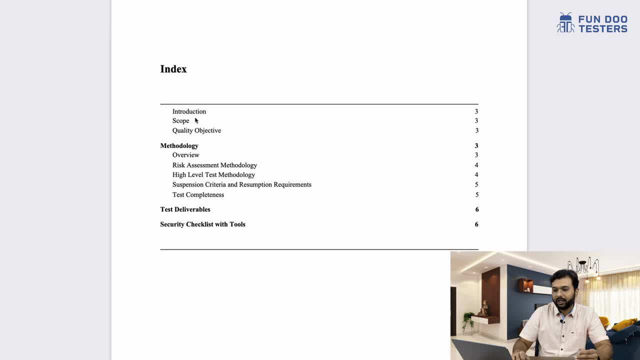 in the test plan. this we are going to mention in the index and index also i have given the hypertext, so if i click on somewhere it will directly navigate to the particular area. so this is how it looks. so second page is a index and third page is a change log. so, based on 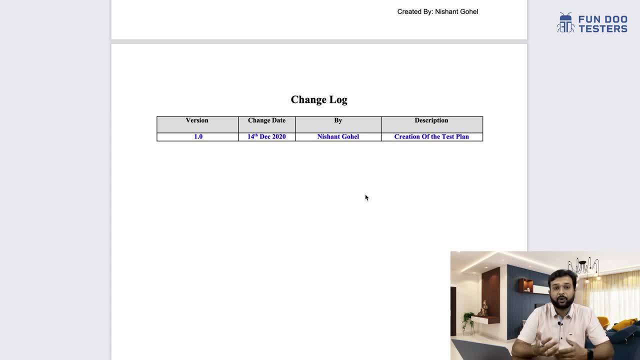 the client requirement or management requirement. we are going to upgrade the document by time by time. so this is we are going to mention in the change log. so this i have created on the 14th december and created by nishant goel, so it's me. and description: creation of the 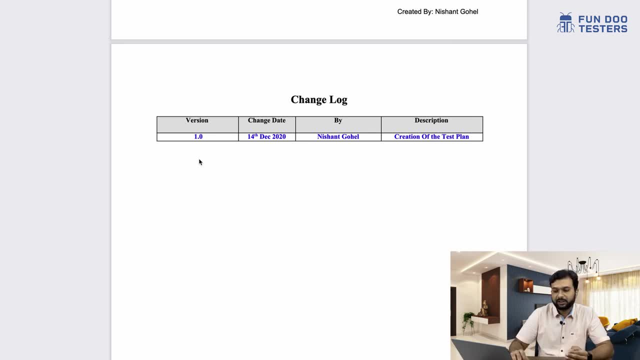 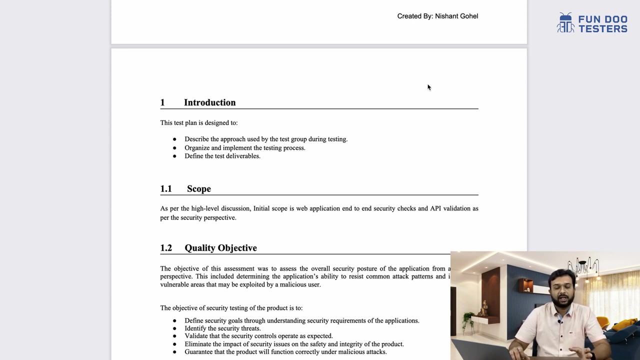 text test plan. so later if we are going to make any changes, then it will be a 2.0 and we have added some section or removed some sections. so we will mention in the description now, first section, as we discussed in test plan, we are starting with the objective, or introduction. 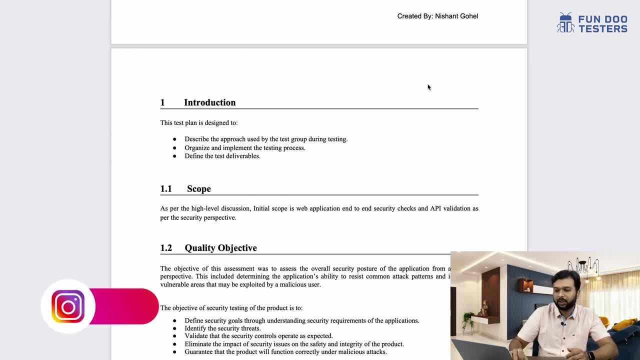 so this will be initial phase, how we are going to start. so here, my first area is an introduction. so introduction means this test plan is designed to. for what purpose you are going to create a test plan? this we have to mention. so i have mentioned. describe the approach used by the. 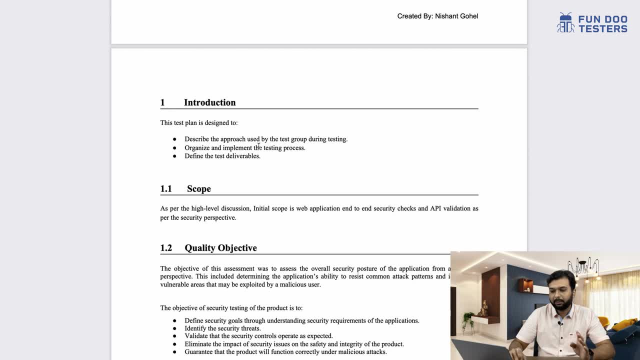 test group during the testing, organize and implement test testing process and defined test variables. so what are the things i'm going to deliver and what are the activities? i am going to do? this all i have mentioned in the test plan. next is a scope. so what is the scope? 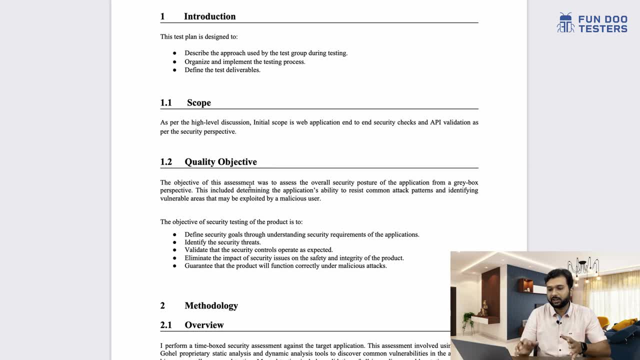 what is high level? things i am going to do that we are going to mention in a scope. so here my high level discuss: yes for the high level discussion: initial scope of the web application: web application end to end security checks and api validation as per the security. 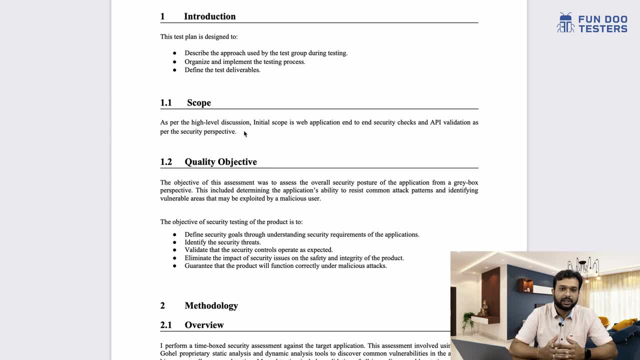 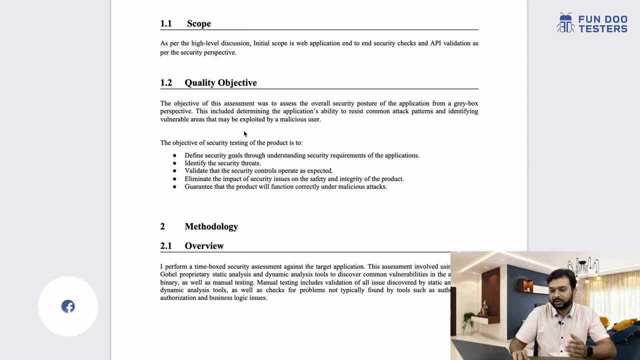 perspective. so i want to perform the security testing i i was planning to by that time. this plan was for a security testing and API validation, so this I have mentioned as a scope, then quality objective, what things we are going to achieve by doing the testing activity. so this I have. 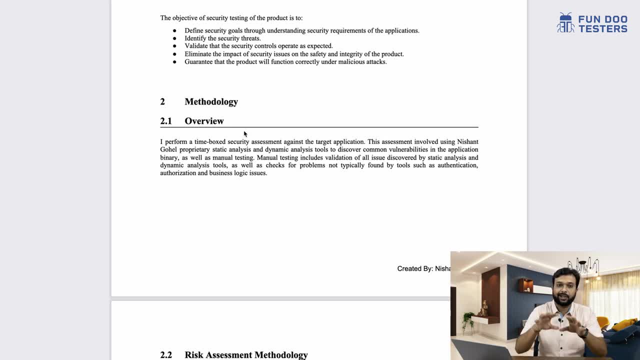 mentioned later on methodology. which methodology? for example, I want to test particular area, let's say big billion day, or I want to test phone pay application. so what will be my objective and how I am going to perform the testing different product? we have to go through the 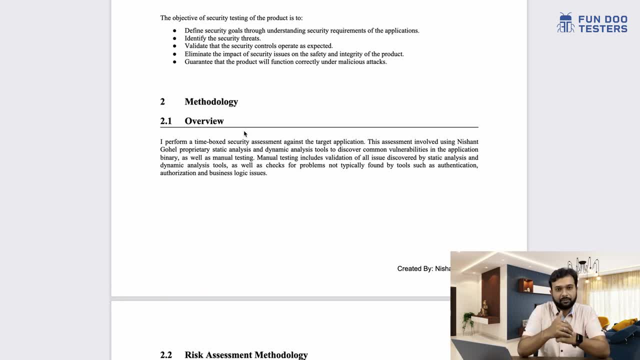 different testing for, let's say, let's take an example of the netflix. so in netflix we have to make sure that whatever we are doing or whatever we are testing, that is up to the mark and when, when end user is watching any movie or any series, they should seamlessly. 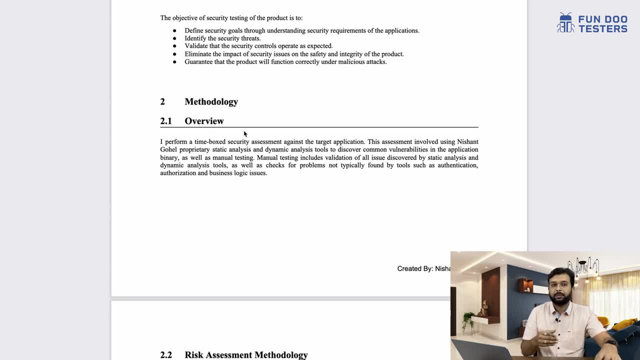 watch the movie. so this will be our aim for the netflix. for example, we are going for a flipkart and they are going to launch a big billion day, so by that time we will go with the performance testing. we are making sure that application will not go down at any point. 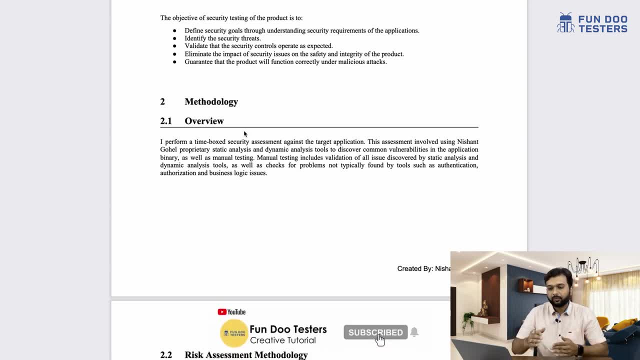 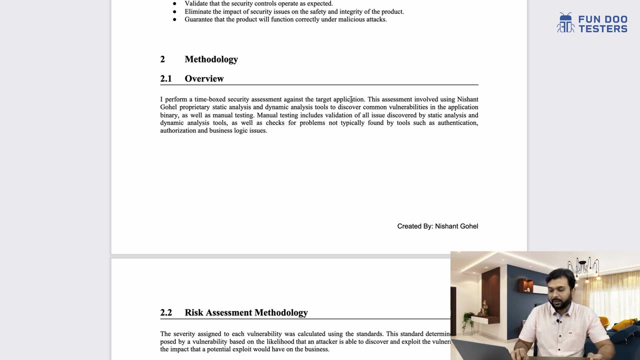 of time by huge load. so similar way, for each and every application we have to define a checklist or methodology which methodology we are going to use. so here I have started. I informed the time I perform a time box security assessment. again, the target application. this assessment involved using the nishant gohel property, static analysis and dynamic analysis. 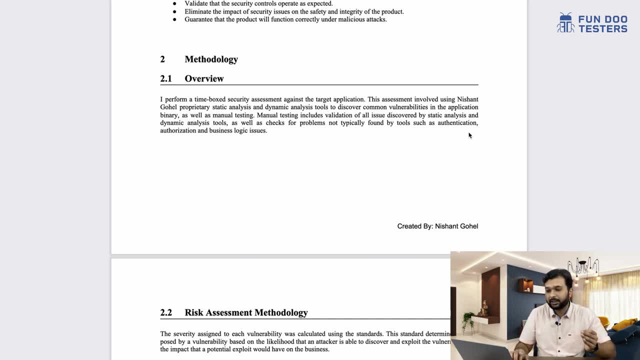 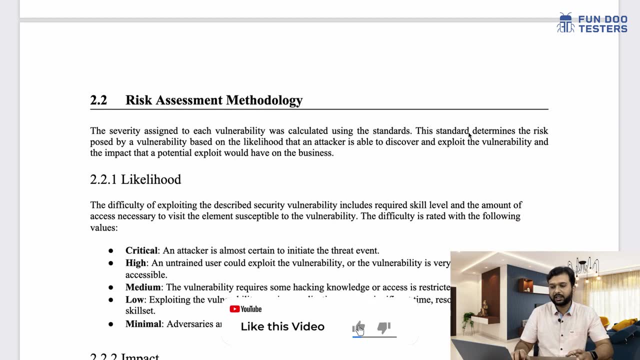 tools to discover common vulnerabilities in the application. so this is what we are going to do, so what I have mentioned, you can pause the video and you can read it out. so now, second thing is risk assessment and methodology. so what I am going to do, what is a critical part? 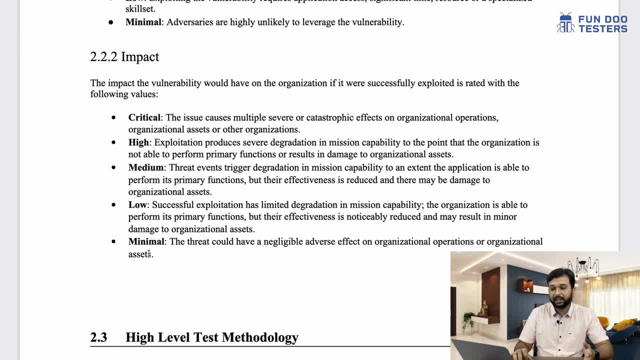 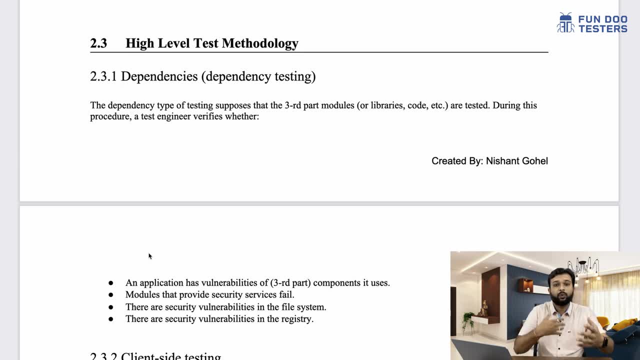 high, high part, medium low and minimal part and what will be the impact? so this I have mentioned later on high level test methodology. so what? I am going to do that because we have to show a clear picture to the client or a management team why we are going to do what. 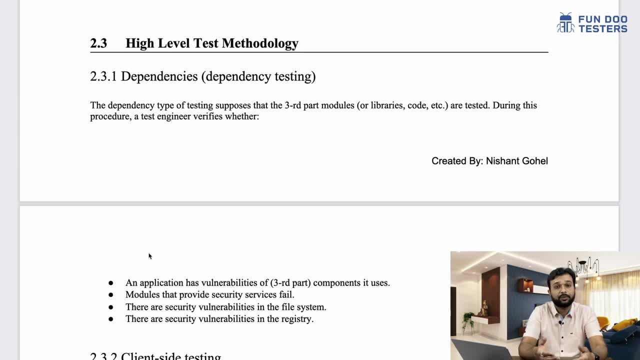 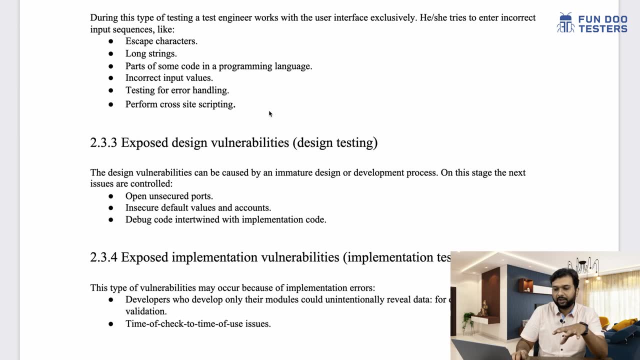 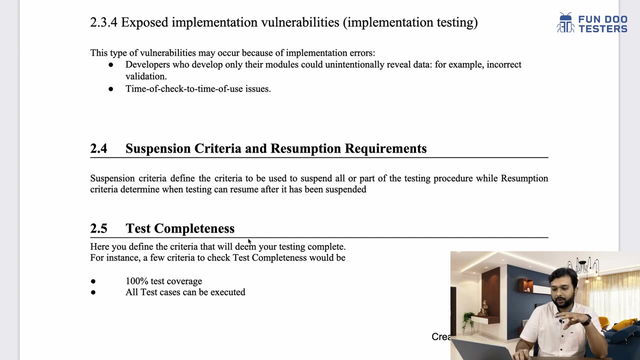 we are going to achieve after it, after it, After completion of the testing phase. so this we have mentioned here: dependency. this is the dependency. I will do the client-side testing. I will find the design vulnerabilities later on suspension or criteria and resumption requirements. so this is again you will read. 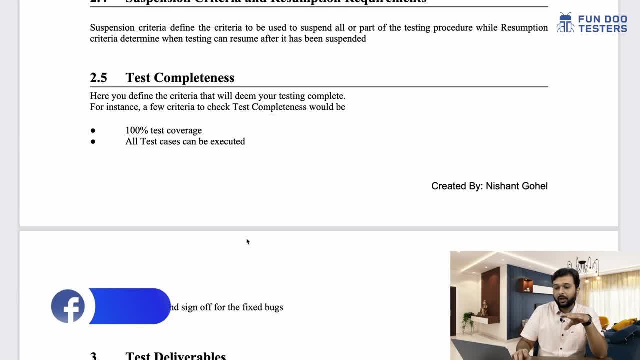 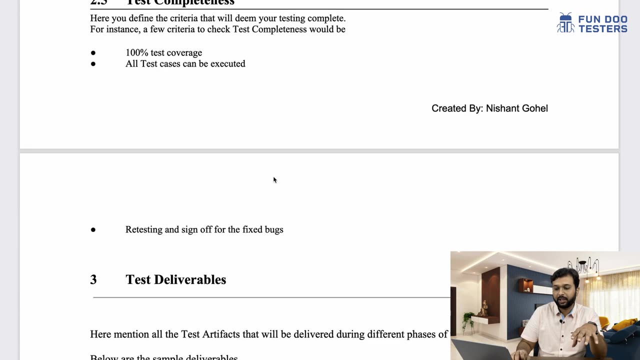 and you will get to know. next is a test: completeness. so here you define the criteria that you will deem your testing complete. so, for example, whenever you are going to complete your test, what will be your criteria? So here I have mentioned 100% of test, test coverage, all test case can be executed, and 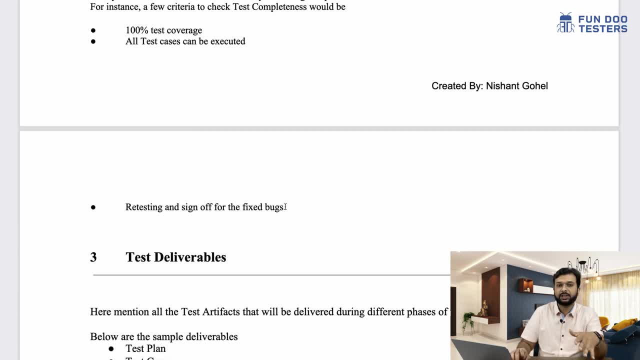 retesting and sign off of the fixed build. so whatever build I am getting, based on that build, I am going to perform all the testing and I will give the sign off. this this will be done from my side, or whatever the let's say we are working for with a huge team. so 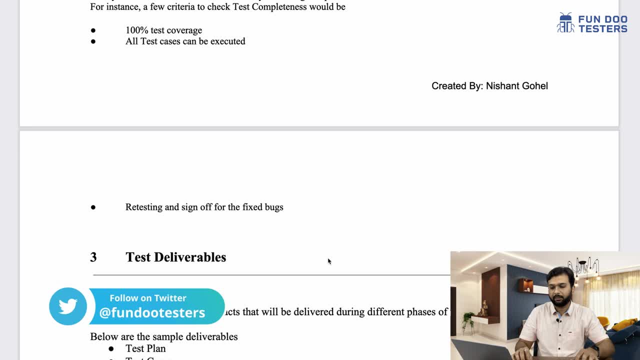 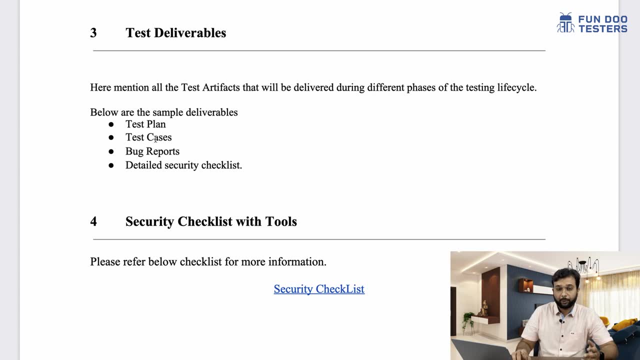 this will be again, collaborative effort from entire team. Next is a deliverable. so this is what I have delivered. let's say I have delivered test plan. I am going to deliver test plan, test cases, bug report and detailed security checklist. so, whatever security testing I am going to do, I will perform all the checklist and you. 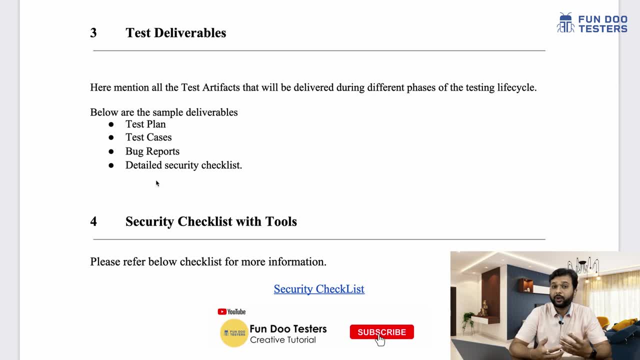 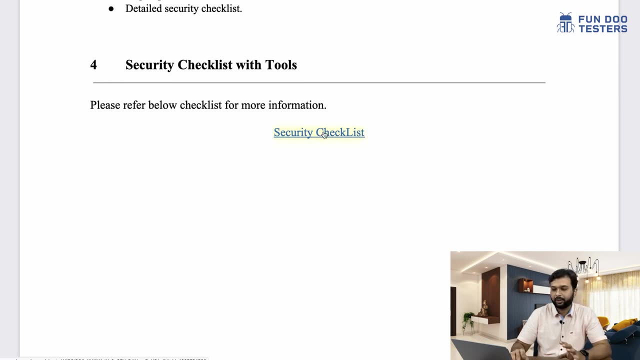 can mention the different mentioned different report. you can attach bug report, you can attach test observation. so all these things we are going to deliver to the client. and here I have mentioned the. please refer to the checklist. I have provided. the checklist I have attached with this document. 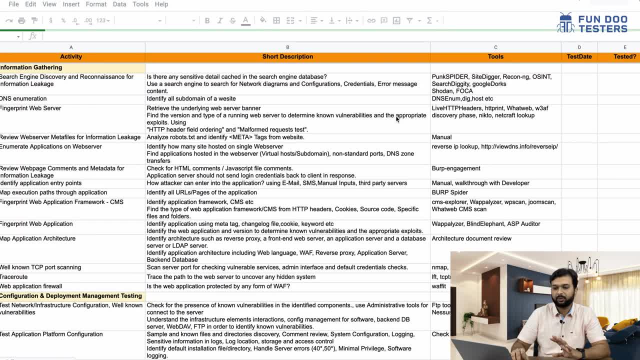 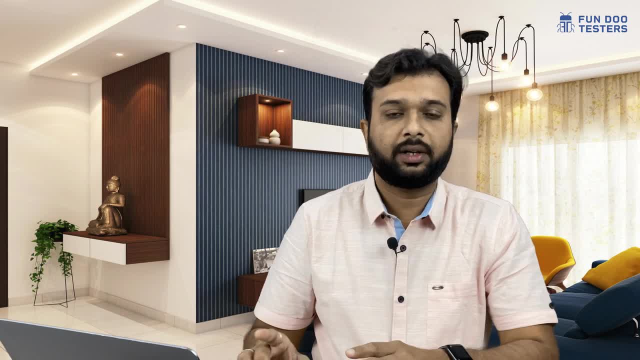 If I am going to click on this, I will be navigated to the entire web application checklist. this is how we are going to create a test plan. I will provide this test plan in a description section. you can read it out so you will get to know what are the things we need to mention. 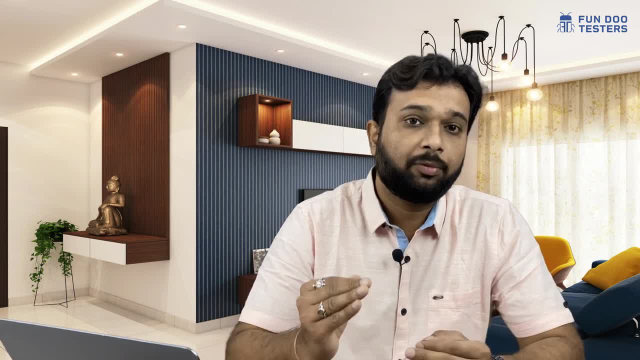 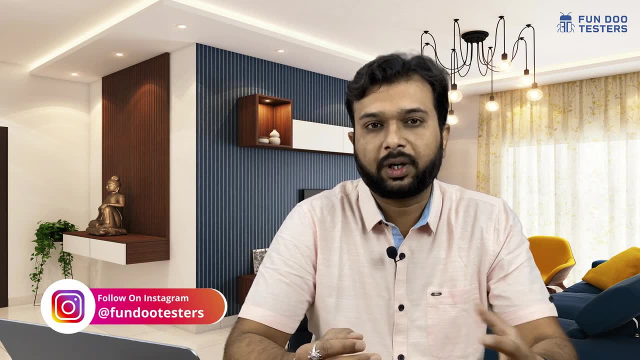 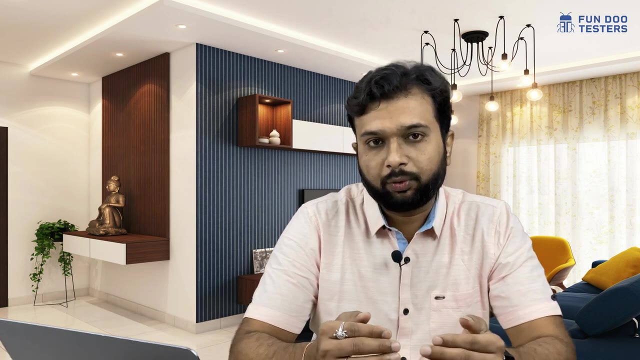 and one more thing. so whenever we are going to create a test plan, by the time we have to show the clear picture. for example, let's say we are looking for some data from the client or management or some other team. So we need to clearly mention: is a blocker part? or if it would be great if you will get?